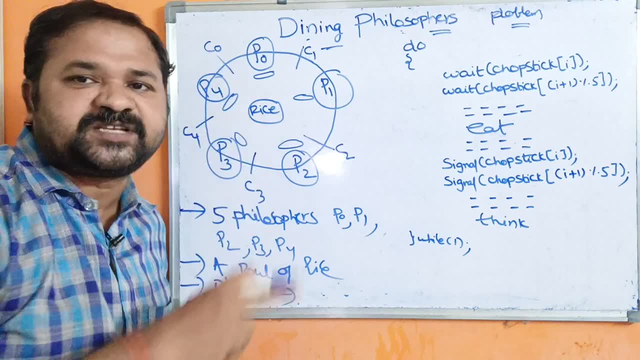 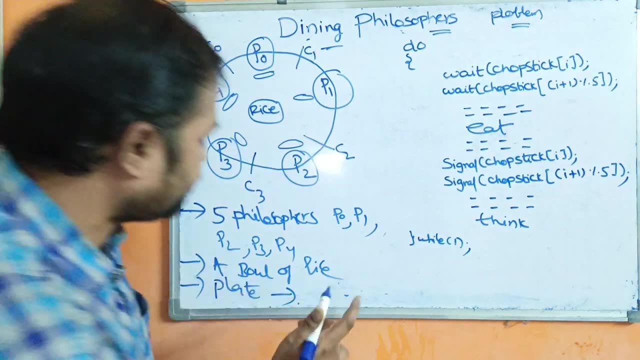 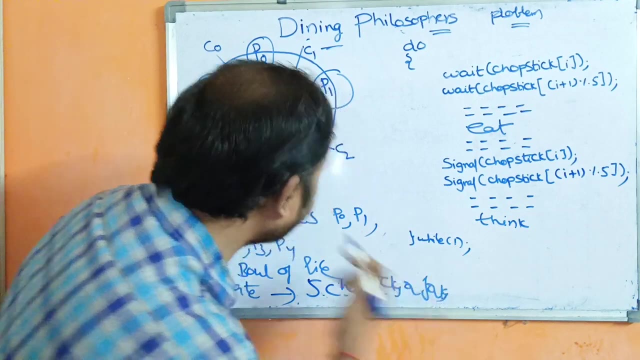 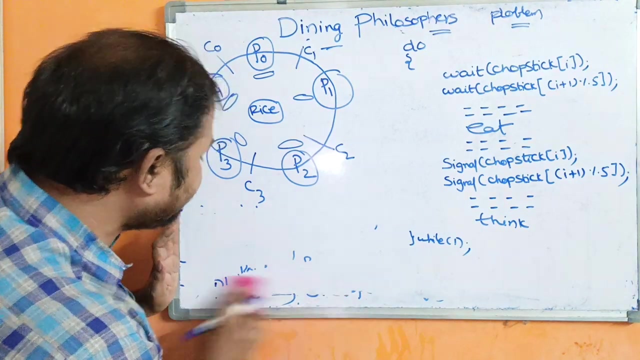 And here 5 chopsticks are there. Chopstick is nothing but fork. Here we are representing chopsticks with the help of C0, C1, C2, C3, C4.. So 5 chopsticks or forks are there Here. each philosopher mainly will be in 2 states. So each philosopher will do mainly 2 activities. 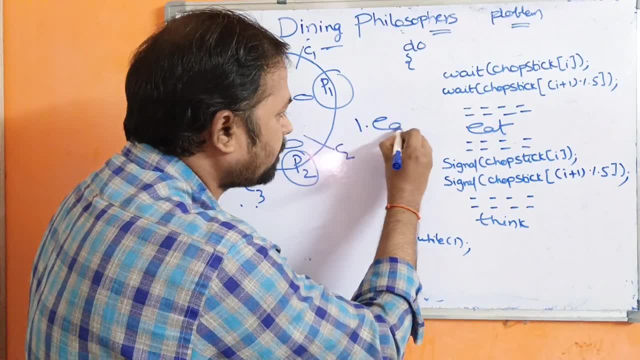 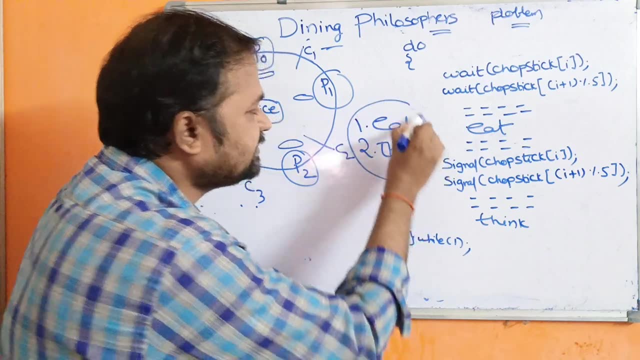 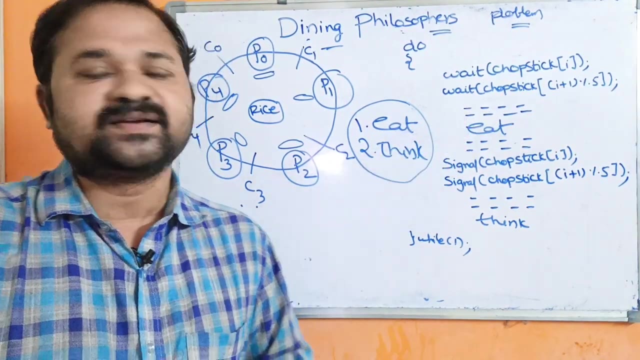 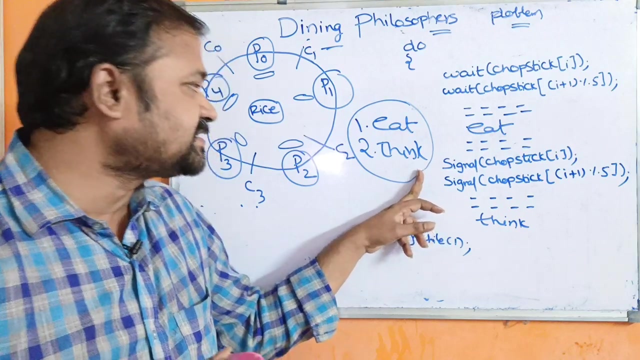 So the first one is: philosopher can eat and the second activity is: philosopher can think. So each philosopher will do these 2 activities. Let us see the first one: If the philosopher is not eating, then it means that philosopher is thinking. If the philosopher is not thinking, then it means that the philosopher is eating. 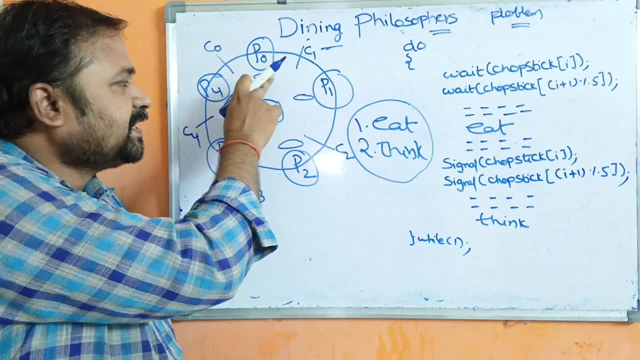 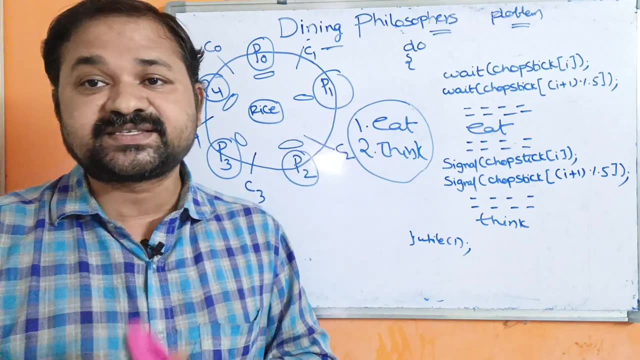 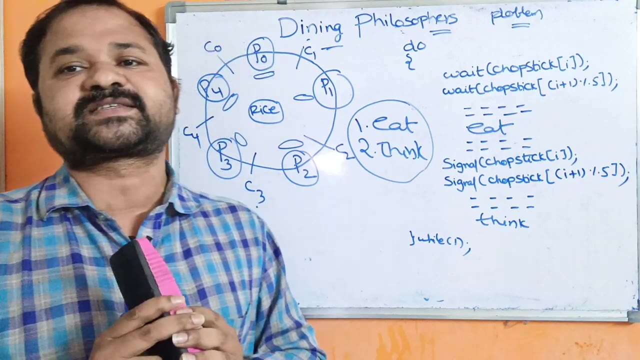 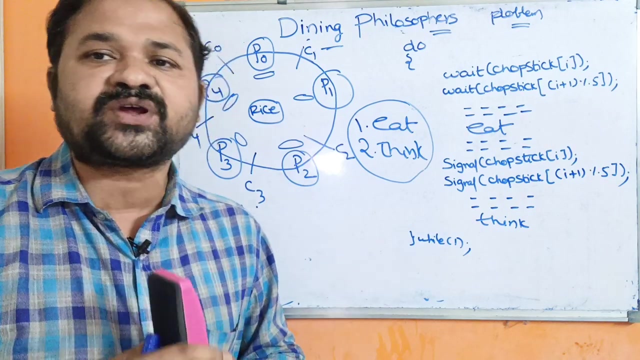 Here P0.. Here, generally for eating, one fork or one chopstick is enough for us. But here the constraint is, each philosopher mainly will be in 2 states. So each philosopher must require 2 chopsticks in order to eat. So on the left side of each philosopher we have a fork and on the right side of each philosopher we have a fork. 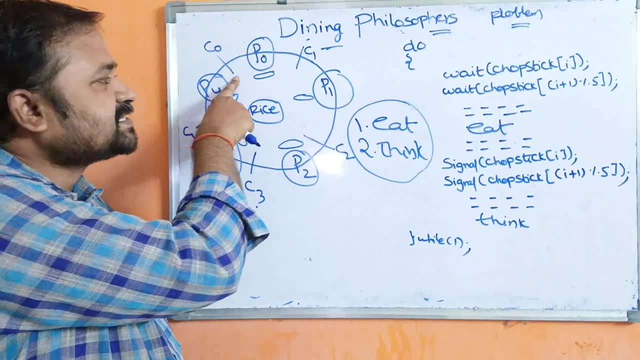 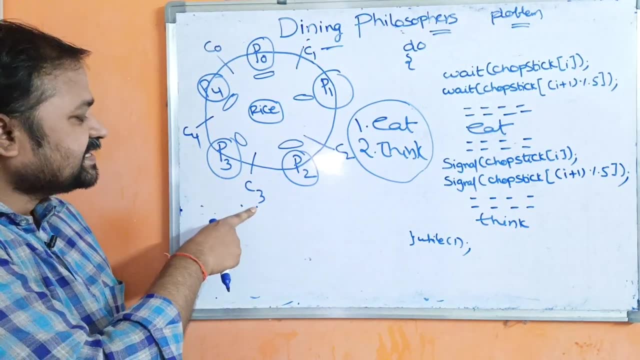 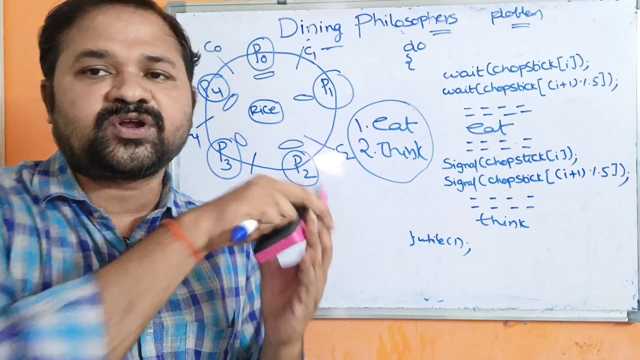 If we consider P0.. So P0 requires C0 and C1 forks for eating. If we consider P3.. So P3 requires C3 and C4 forks for eating. So each philosopher must require 2 forks, So one fork on the left hand side and another fork on the right hand side in order to eat. 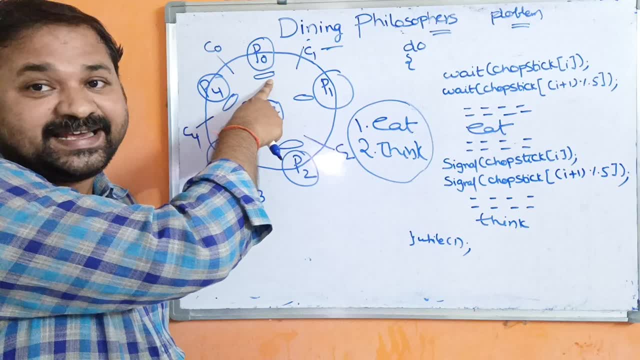 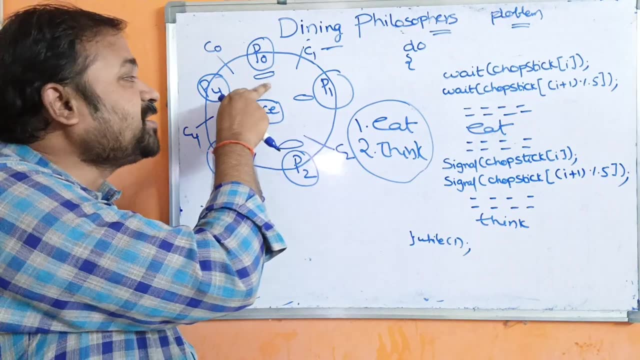 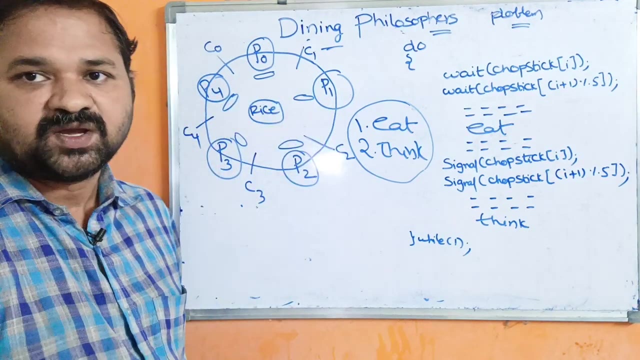 Assumes that P0 is eating, So P0 is eating means P0 grabbed C0 fork as well as C1 fork. Assumes that P0 is eating, Then we can say that there is no chance for P1 and P4 to eat. 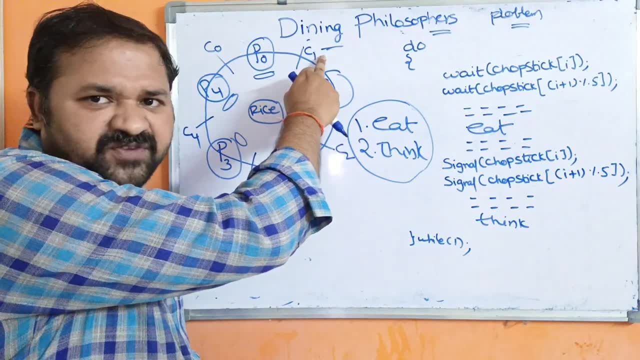 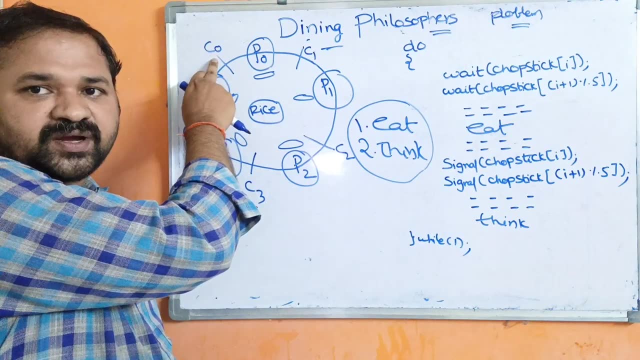 Why? Because in order to eat, P1 requires C1 fork, But C1 fork was not enough, So P2 was acting. And when C2 was acting, So P1 was acting. So P2 was acting, already acquired by P0.. If you consider P4, P4 required C0 fork, but C0 fork was already acquired. 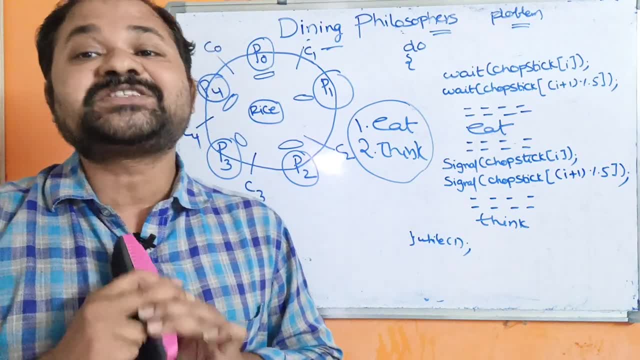 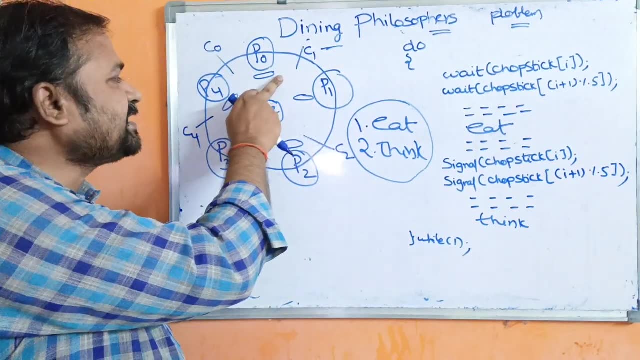 by P0.. So here the point is: it is not possible for the adjacent philosophers to eat simultaneously, So while P0 is eating. so it is not possible for P4 and P1 to eat While P0 is eating. 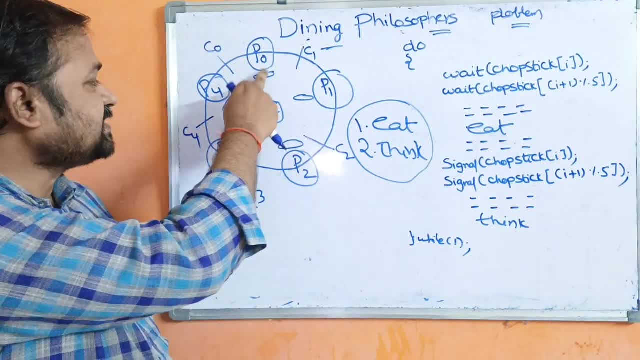 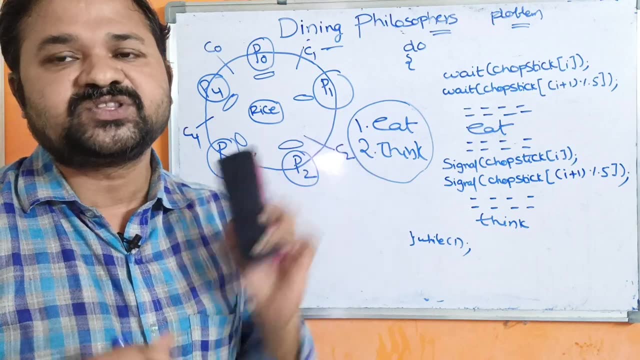 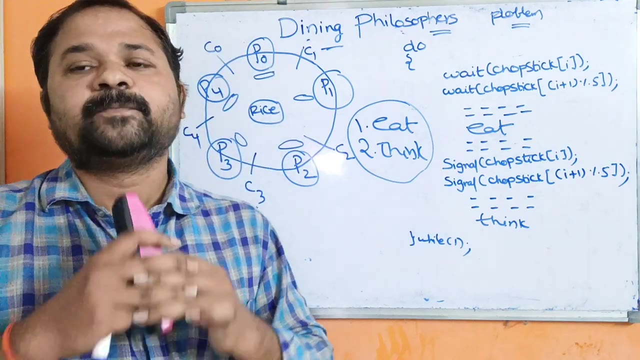 then there is a chance for P2 to eat. Likewise there is a chance for P3 to eat, But adjacent philosophers cannot eat simultaneously. So this is the problem here And here. one more problem is suppose: assumes that all the philosophers becomes hungry simultaneously. 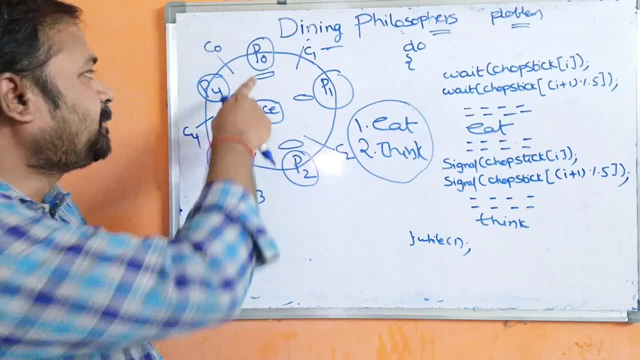 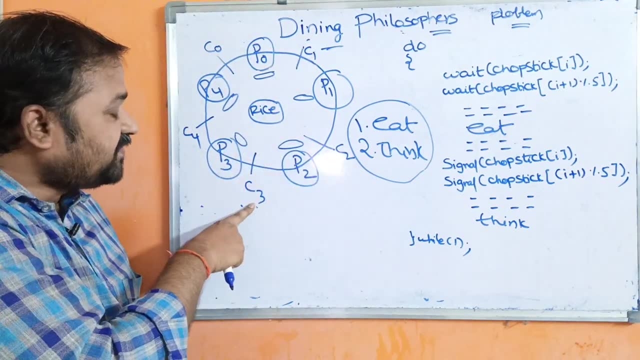 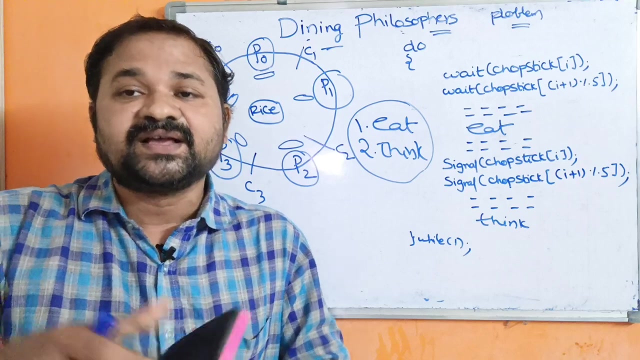 and each philosopher get one fork. Let P0 acquired C0 fork, P1 acquired C1 fork, P2 acquired C2 fork, P3 acquired C3 fork, P4 acquired C4 fork. So now what will happen? Each philosopher will wait for another fork, But that fork was already allotted to some. 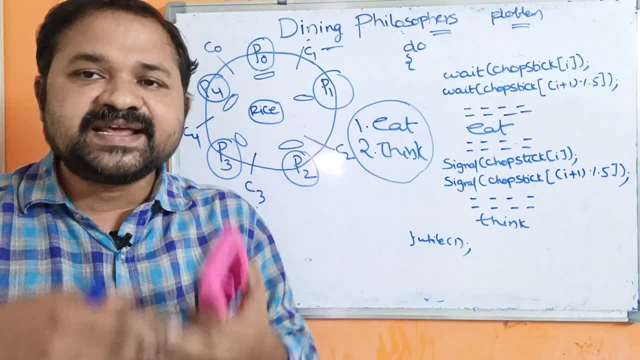 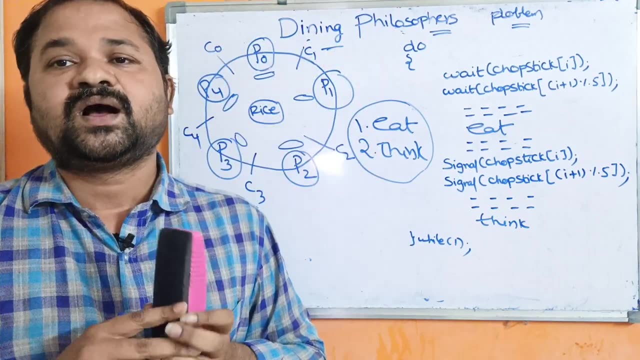 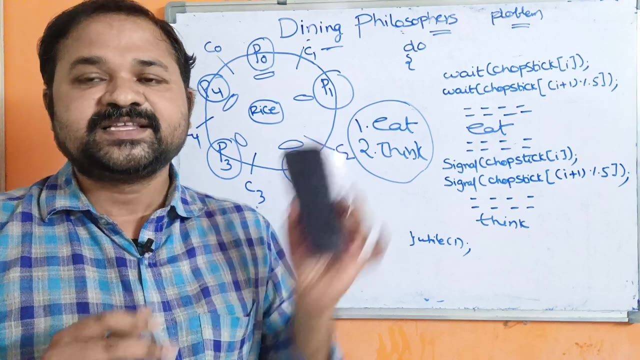 other philosopher, So likewise each philosopher. there is a possibility that each philosopher may wait for that chopstick for a longer period of time And then, because of starvation or hungry, a philosopher may die. So that is the problem here. This problem is called as: 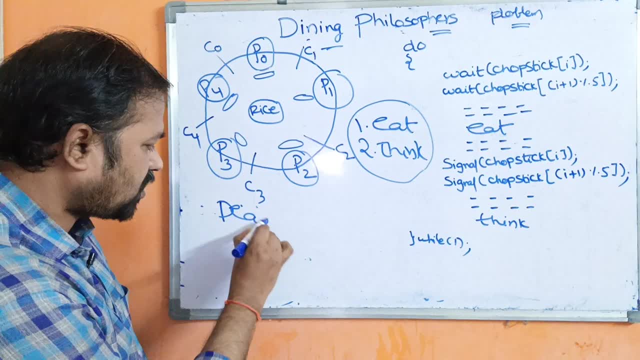 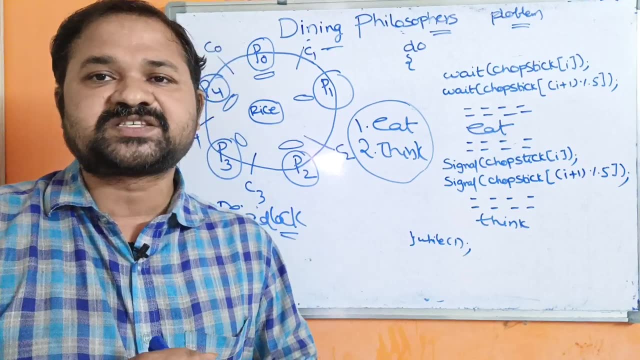 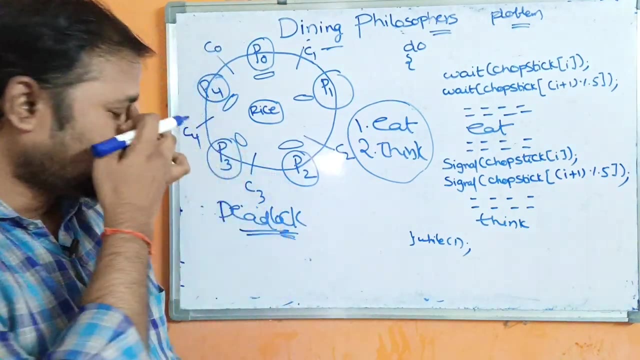 deadlock problem. So this problem is called as deadlock. Why? Because each philosopher need another fork, but that fork was already allotted to some other philosopher, So likewise, each philosopher has to wait for a longer period of time, So a deadlock may occur here. 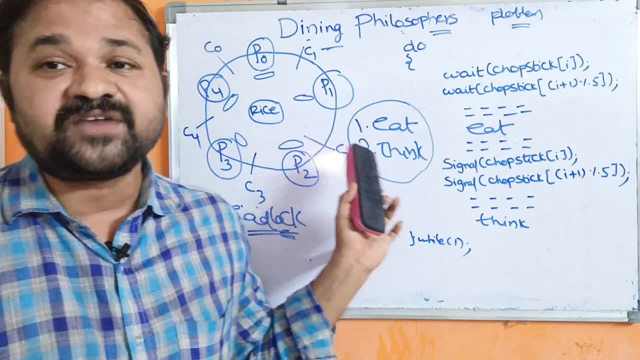 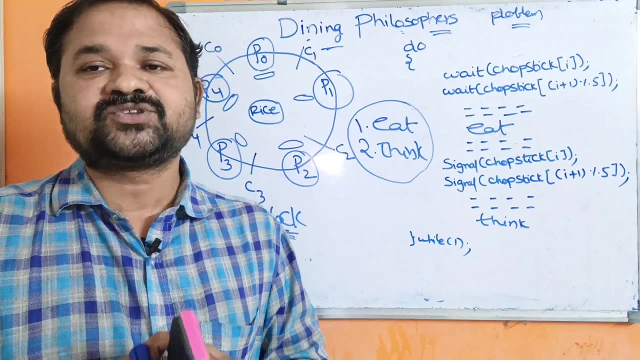 How we can solve that problem. Here, our target is: with starvation, no person has to die. That means each philosopher has to get a chance for eating. So that is the problem here. So how to solve this problem? In order to solve this problem, we are using this algorithm. 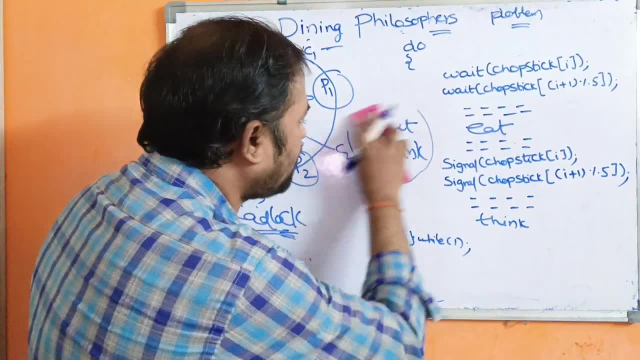 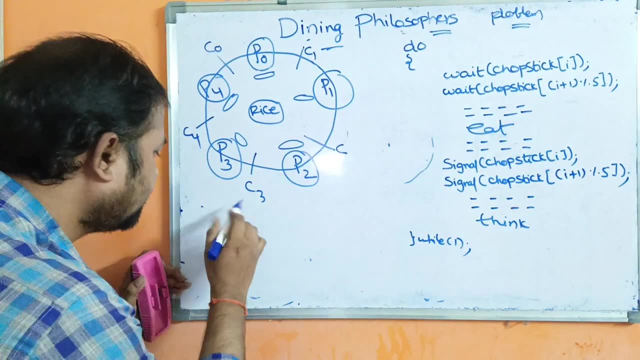 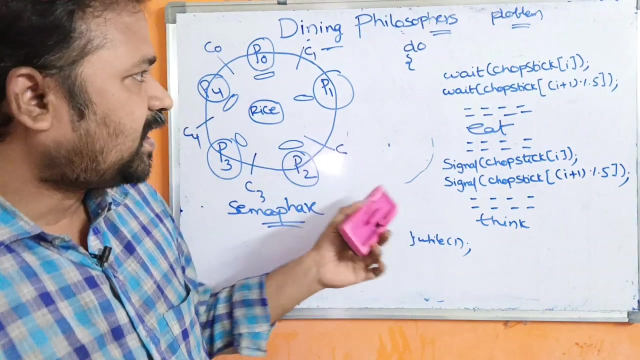 Here we are implementing this algorithm with the help of a semaphore. So we know what is a semaphore. Semaphore is nothing but an integer variable Semaphore. here we are using binary semaphore. Binary semaphore means the value may be either one or zero. Here the semaphore 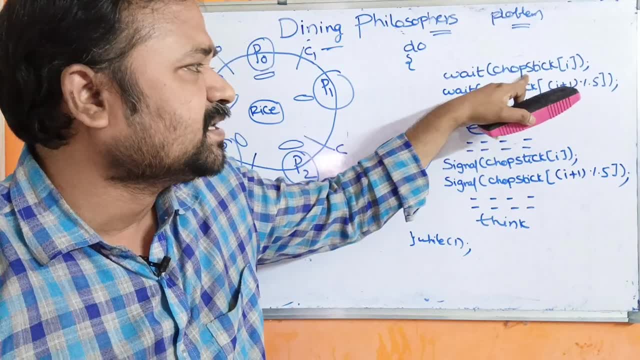 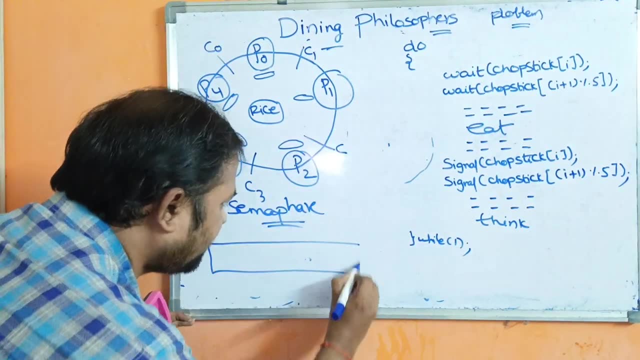 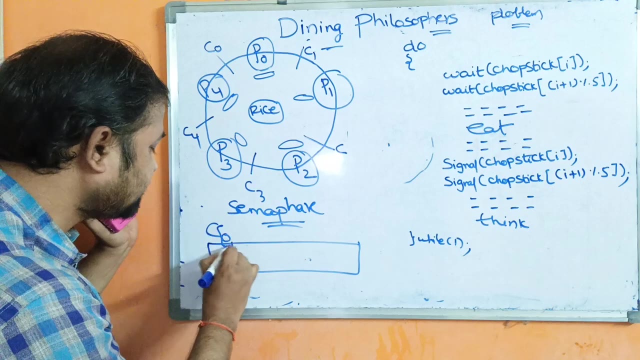 is represented with the help of chopstick variable. Here chopstick is nothing but an array. So here, totally, we have: how many philosophers are there? five philosophers are there. so here this is nothing but a semaphore array variable. so first chopstick is c of 0, next one is c of 1, next c of 2, so totally five persons are there. 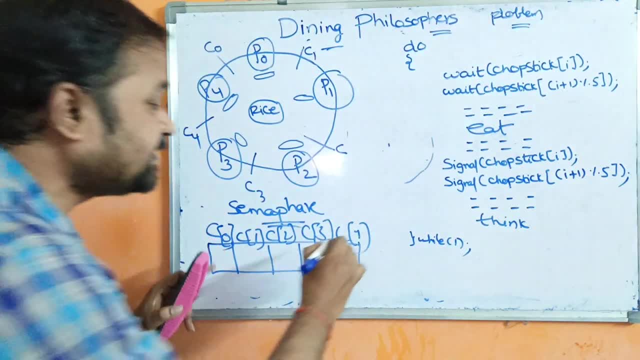 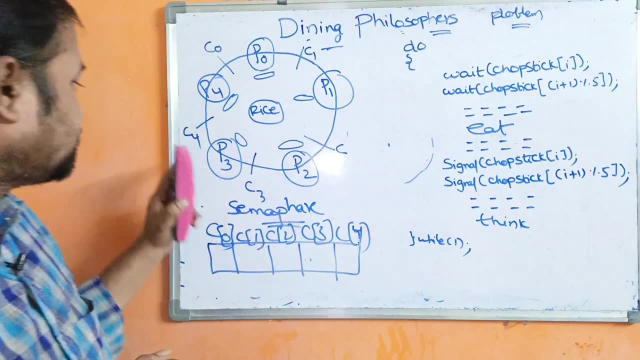 so c of 3, c of 4, where c of not represents the first chopstick, that is nothing but c. not if we consider c of 3. c of 3 means fourth chopstick, so that is nothing but c of 3. okay, here let us assume. 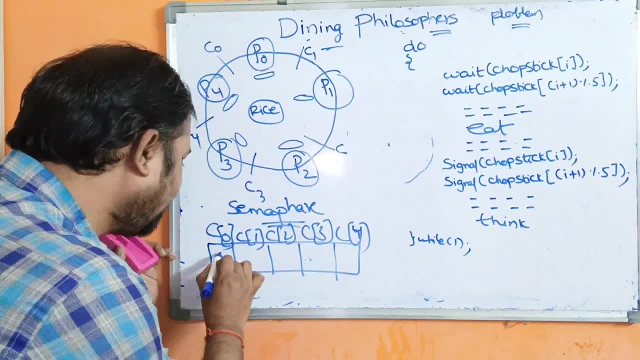 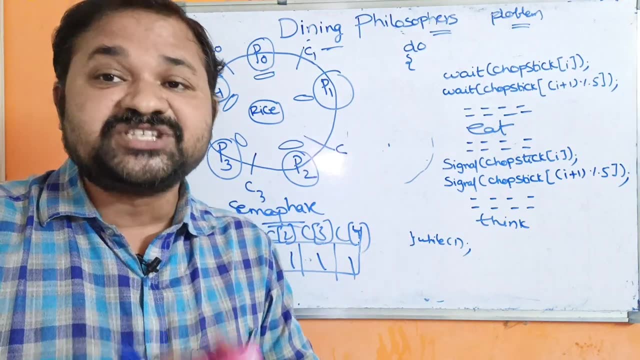 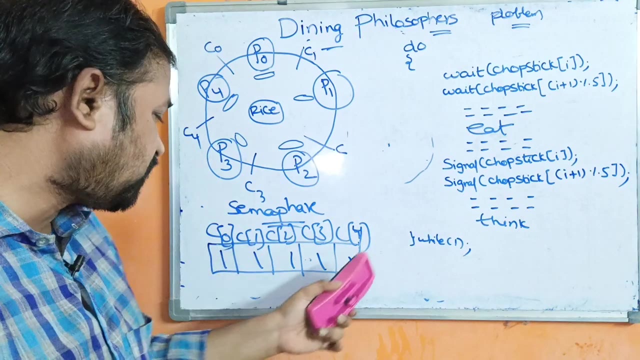 that initially all these chopsticks contains an element called 1. so here 1 means that the chopstick is free, whereas 0 means that the chopstick was already allocated to some other philosopher. here all initial values of all these values are 0- 1 why? because initially all the 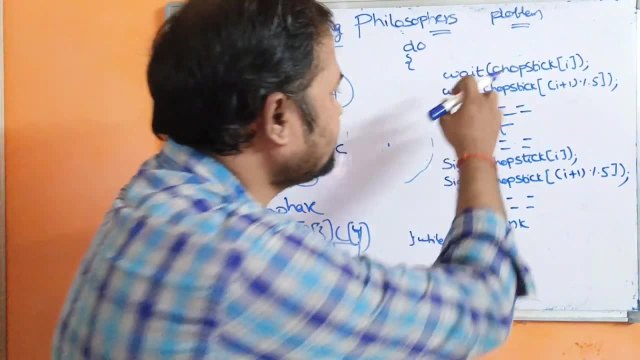 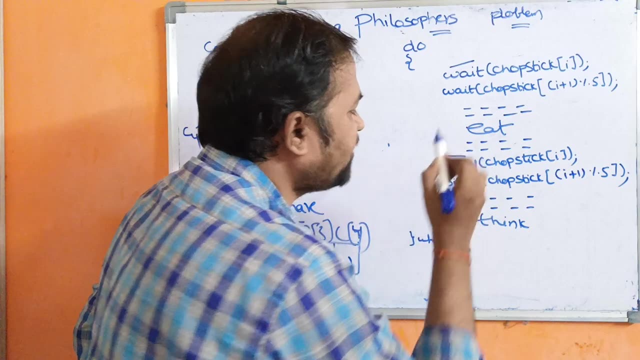 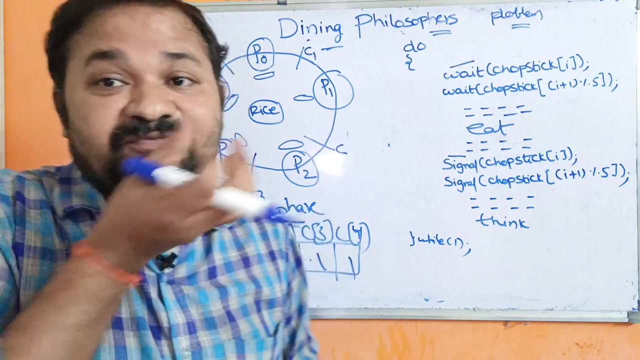 chopsticks are free here. so this is the function here. here, mainly, we are using two operations. the first operation is weight operation. the second operation is signal operation. first let's see what is weight operation. a philosopher can get a fork, a chopstick with the help of the weight operation. 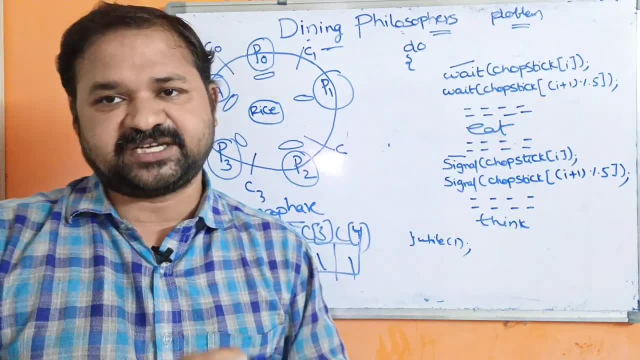 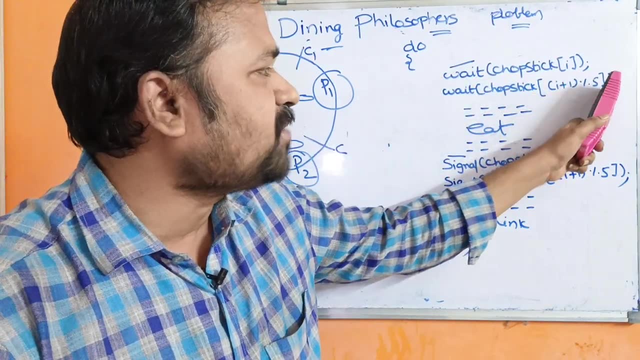 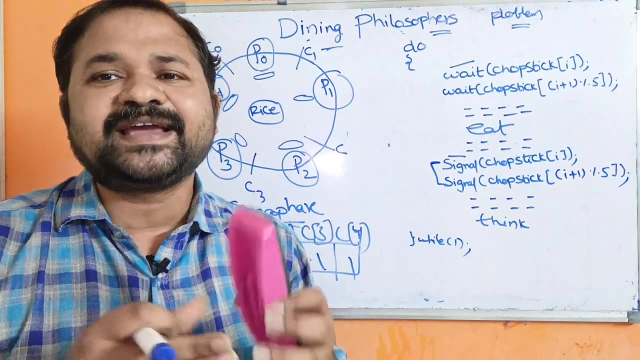 so weight of chopstick of i means first chopstick. he will get the first chopstick with the help of this operation. weight of chopstick of i plus 1 modulo 5 means second chopstick. okay, and next of these operations will be the seating operation. so once the eating is over, then the philosopher. 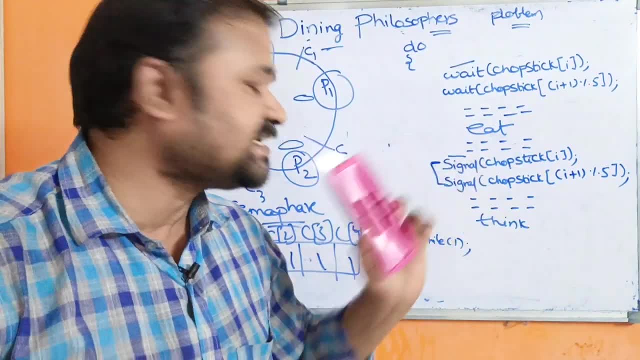 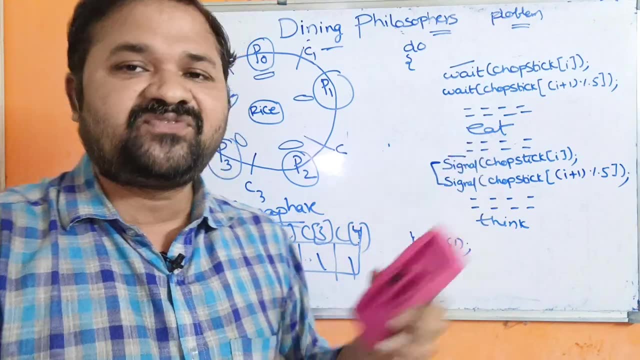 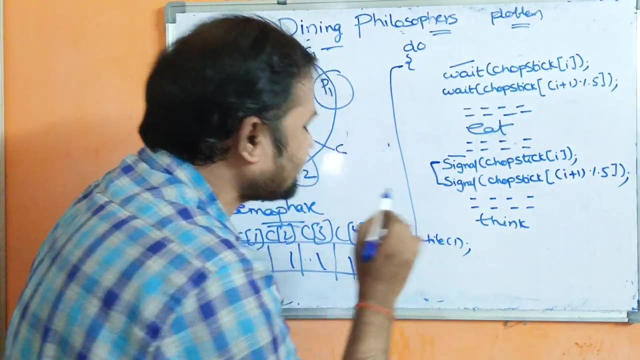 has to place that chopstick or fork on the table with the help of the signal operation. so mainly we are using two operations. so wait for grabbing the chopstick and signal for placing the corresponding chopstick on the table. now let us assume that p not has executed weight operation first. so what is the operation? weight of chopstick of i. 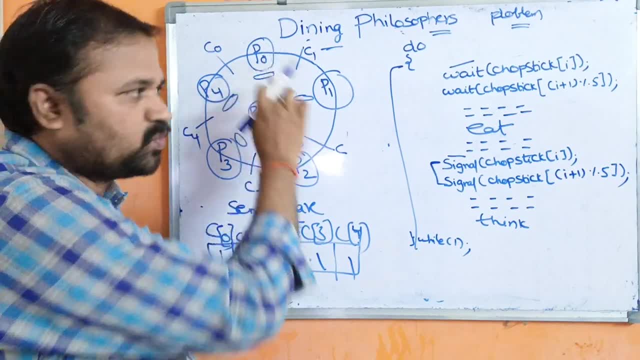 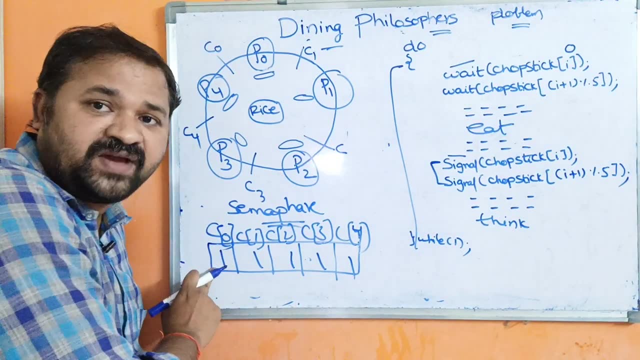 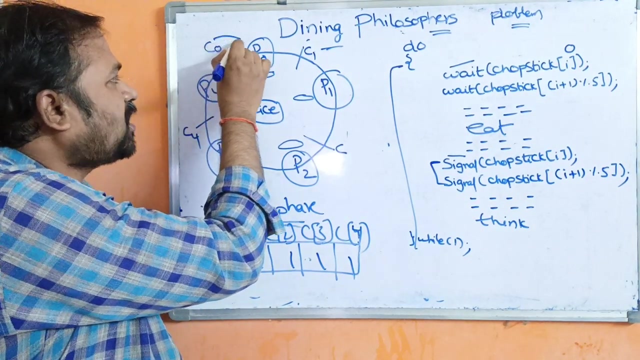 so here p naught means, here the number is zero. so weight of chopstick of zero: weight of chopstick of zero, that means c of zero. so what is c of zero? value one, so one means that it is free, c zero is free. so now c zero will be allotted to p naught. and here c naught is allocated, so one is changed. 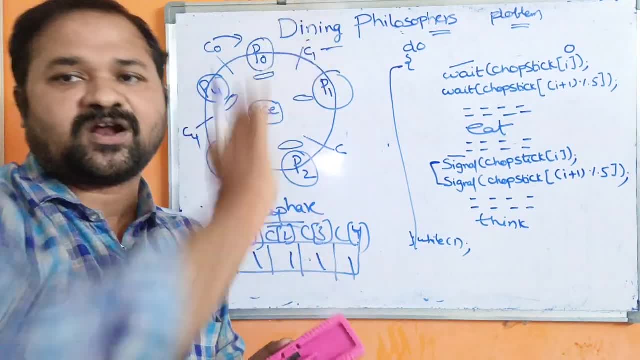 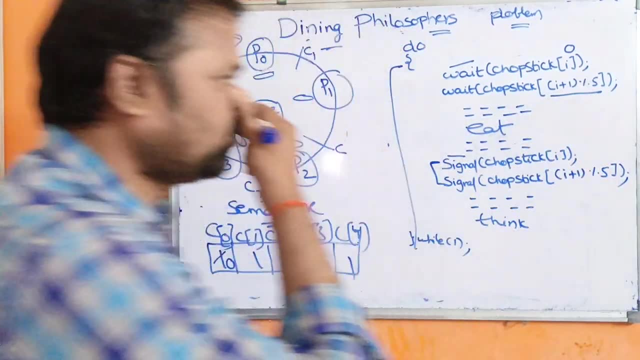 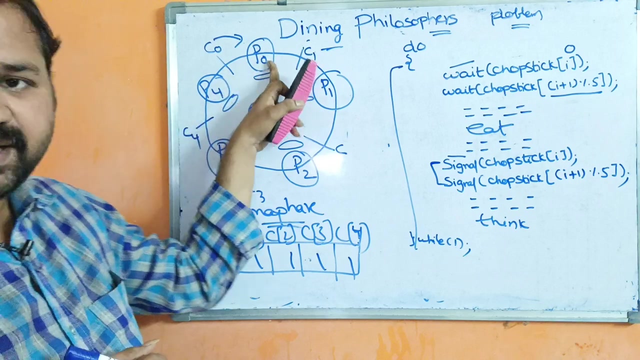 to zero. so zero specifies that that chopstick was allotted. okay, next, weight of chopstick of i plus one modulo five. so this is nothing but circular q. okay, here we have p naught, p one, p two, p three, p four. so after p four we have p naught. so in order to go from c four to c naught, we are: 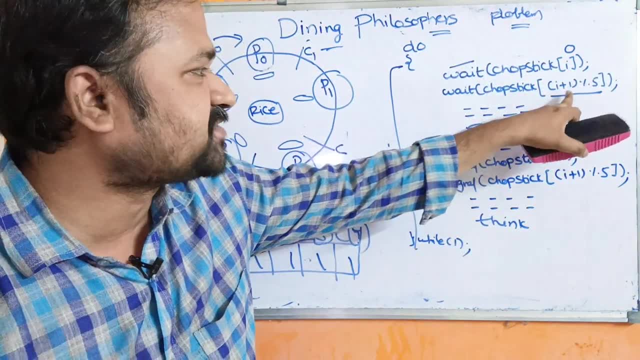 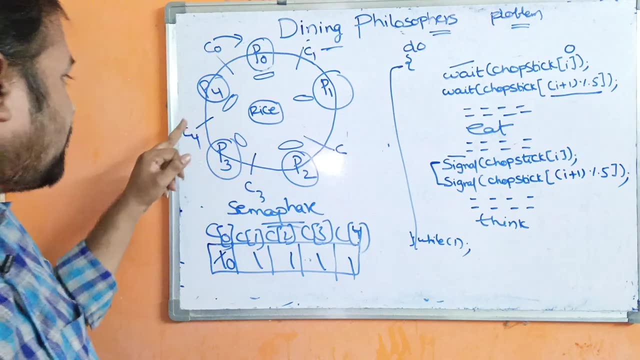 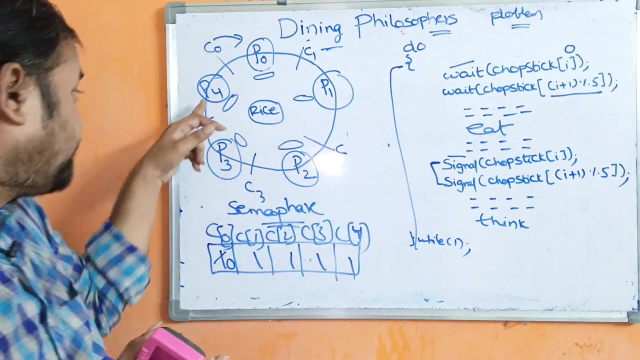 using this, this one, this function. so i plus one. so let us assume that i value is four. so four plus one means five. five mod five means zero. so from four we can go to zero with the help of this function. this is nothing but circular q implementation. from p four we have to go to p. naught, okay, so that should be. 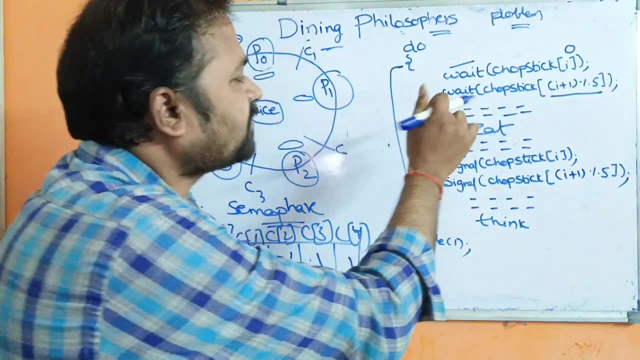 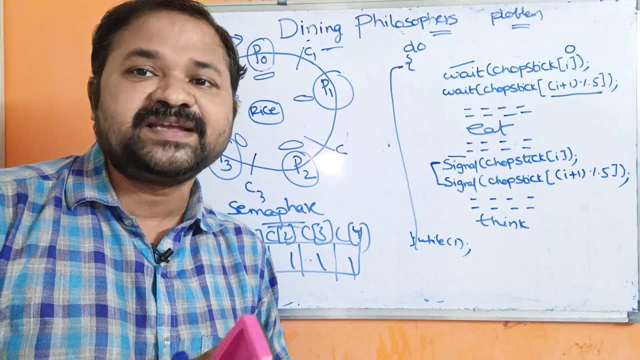 done with the help of this function. okay, next p naught will execute this operation. weight of chopstick of i plus one here. what is i value? zero? so zero plus one means one. one modulo five means one. modulo five means five. ones are five, zeros are zero. 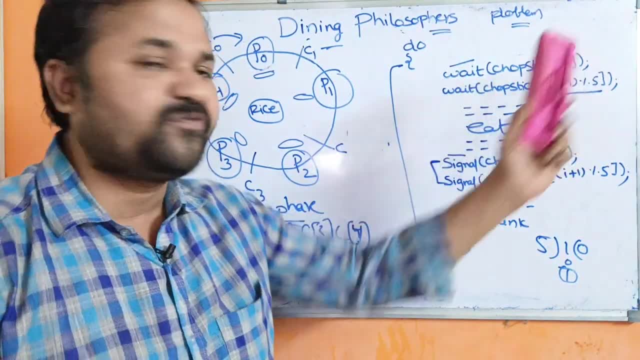 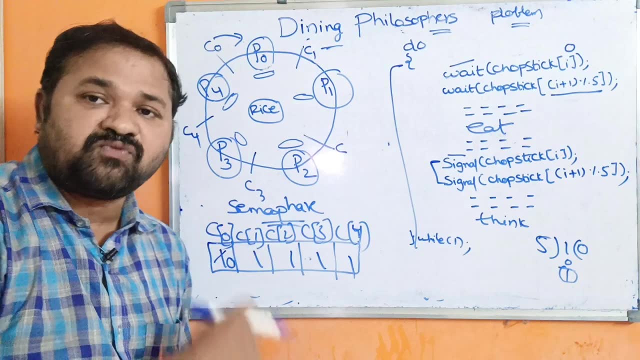 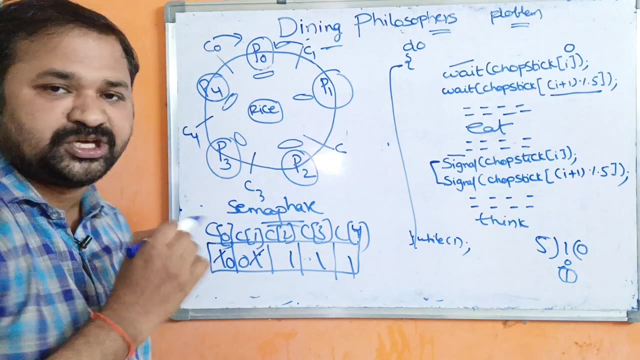 one so one. modulo five means one, so weight of chopstick of one. that means here weight of c of one, so one so one. it means that c of one is free. so now it now c of one will be allocated to p naught. so this value will be changed to zero. now why? because it was c one fork was allotted to p naught. 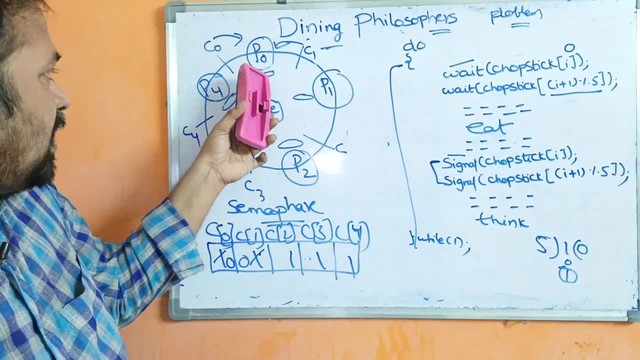 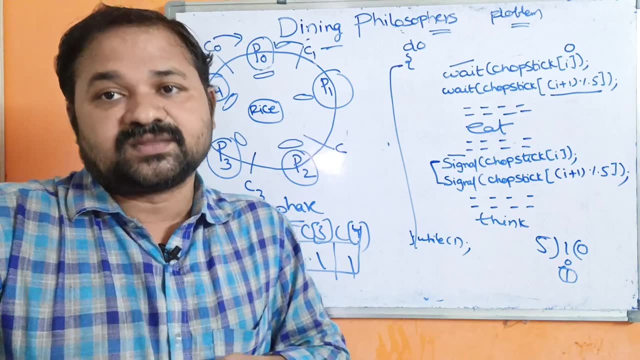 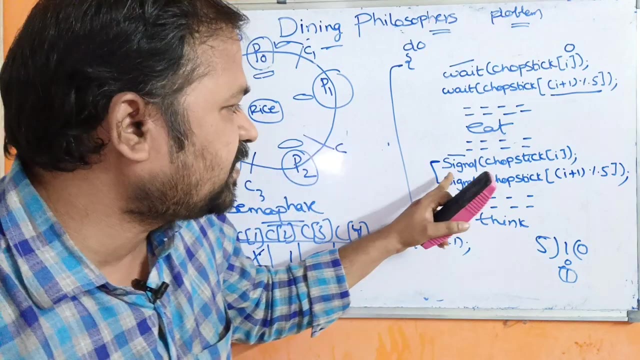 okay, then after that p naught will use c naught and c one fork for heating. so one, the heating is over. then p naught, philosopher, philosopher. one has to put down the corresponding forks on the table. so for that purpose, signal operation is implemented. signal of chopstick, of i. 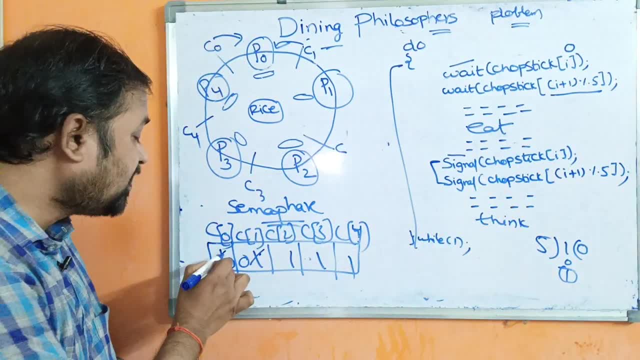 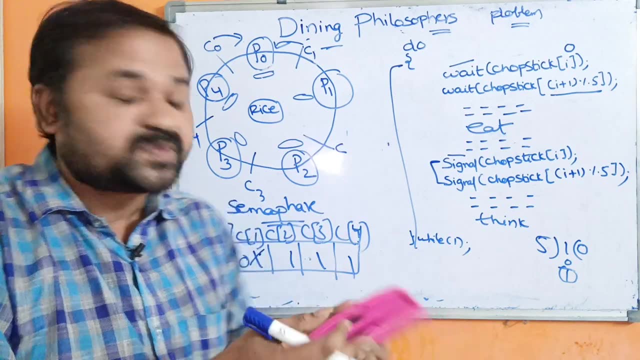 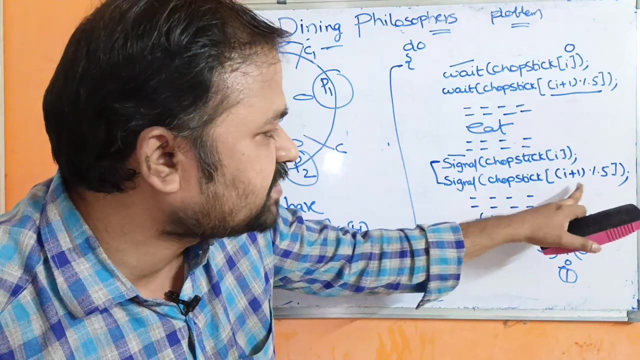 signal of c of zero. c of zero. signal operation means: uh, here that person is placing the chopstick on the table. so now the chopstick is free. so now this zero will be changed to one. okay, this zero will be changed to one. then, after that, signal of chopstick of i plus one modulo five. so zero plus one means one, one modulo five. 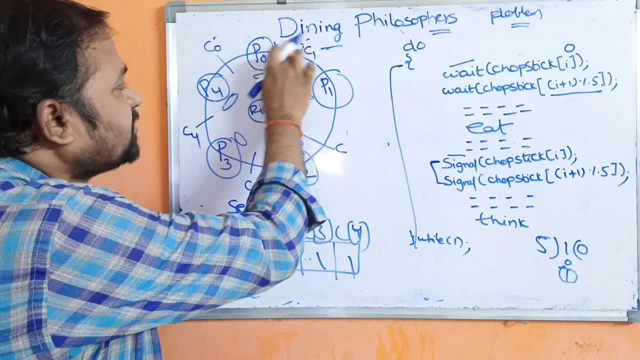 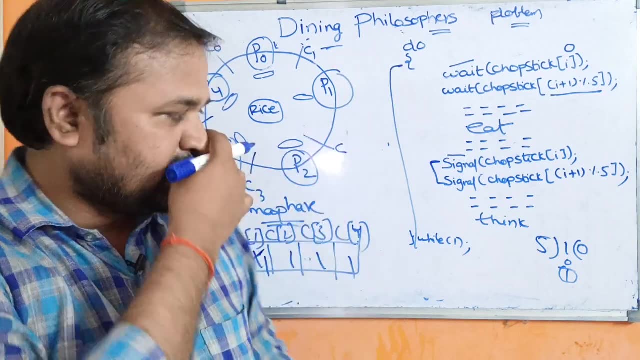 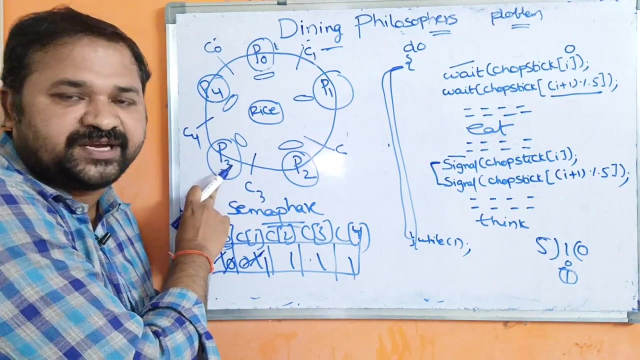 means one so. so now c one is also free, so c one is also free, so one one. all the values are one, so likewise any philosopher can execute this algorithm. let us assume that p3 wants to eat. p3 wants to eat, so first p3 executes weight of chopstick, of what is i value. p3 means here the. 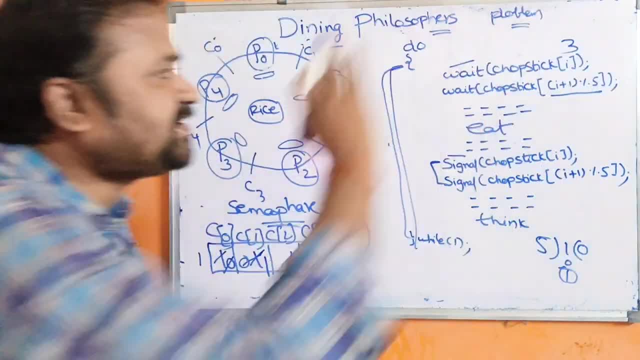 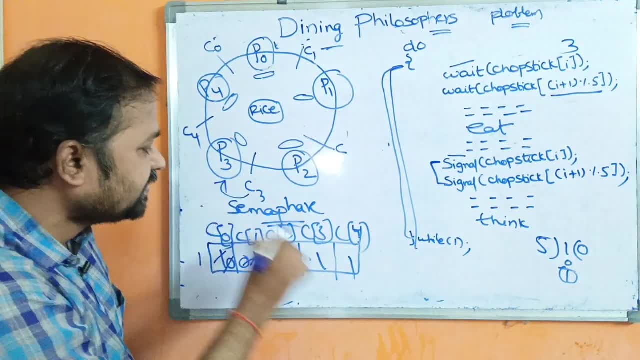 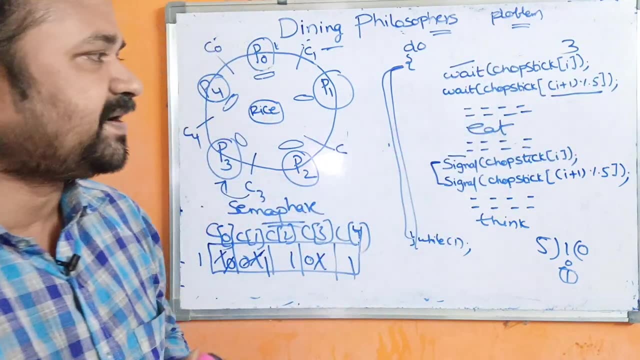 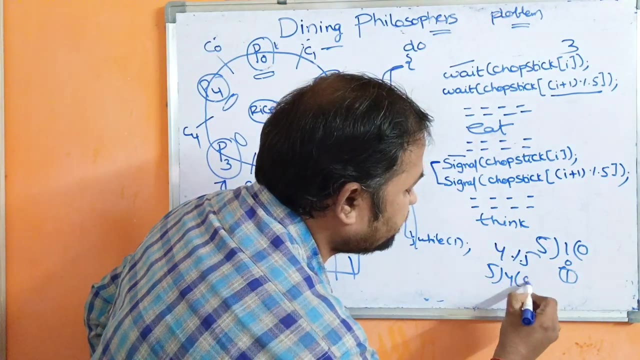 so now c of three will be allocated to p3, so this value will be changed to zero. okay, next the pillow, next weight of chopstick of i plus one modulo five. so three plus one means what four, four modulo five means four. modulo five means what five, four, five zeros are zero, four minus. 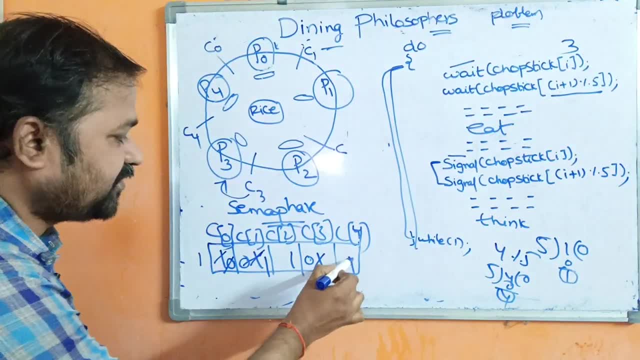 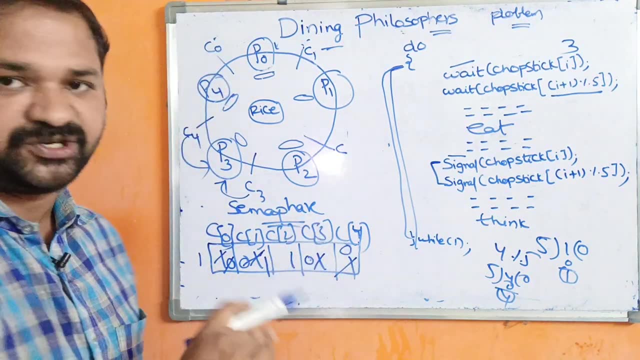 zero means four, so c four, c four is also free here. okay, so now this c four fork will be allotted to p3. so here it is not free now, so it is changed to zero. okay, so now p3 got c3 and c4 folks. so with the 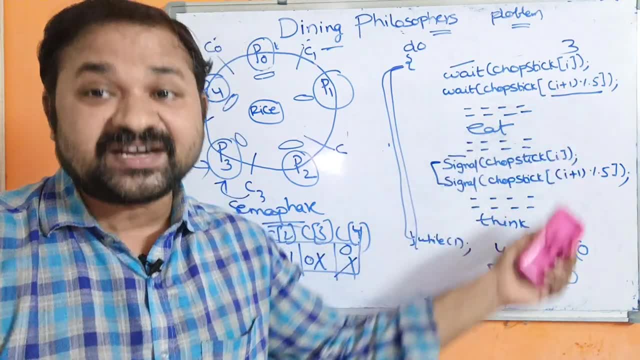 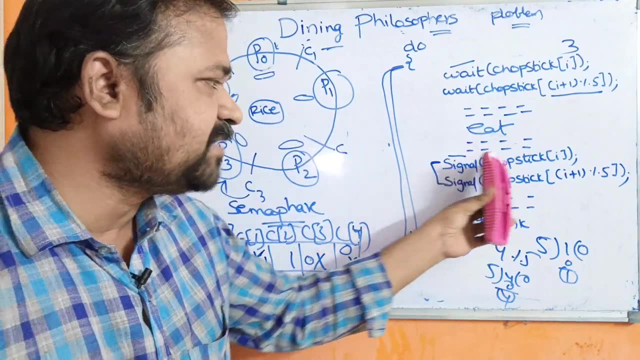 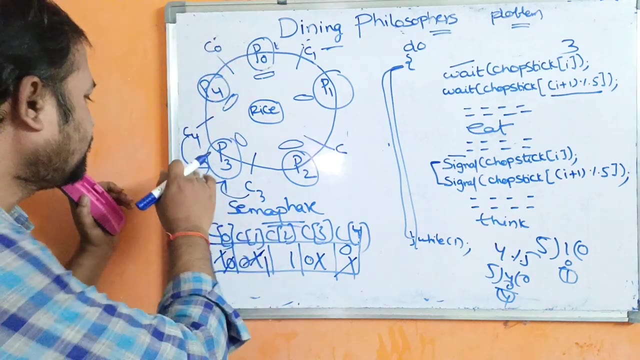 help of those two folks. p3 can eat now. after the eating is over, then p3 has to put down the corresponding two folks on the table. so that should be done with the help of the signal operation. so signal of chopstick of i. here the index is three, so signal of c of three. so now what will happen? the c of three value. 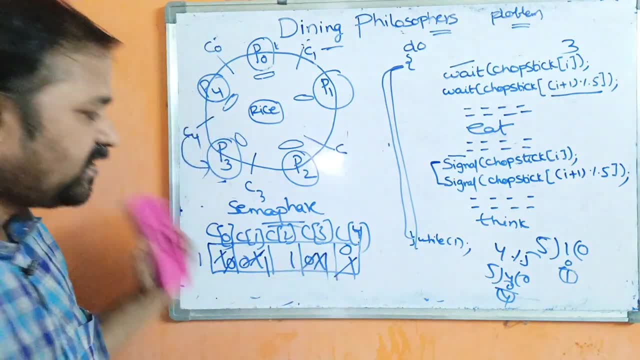 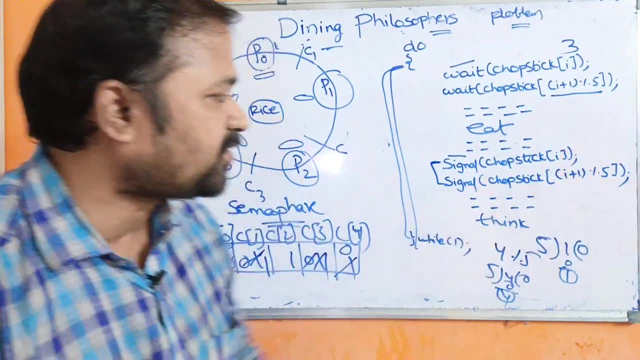 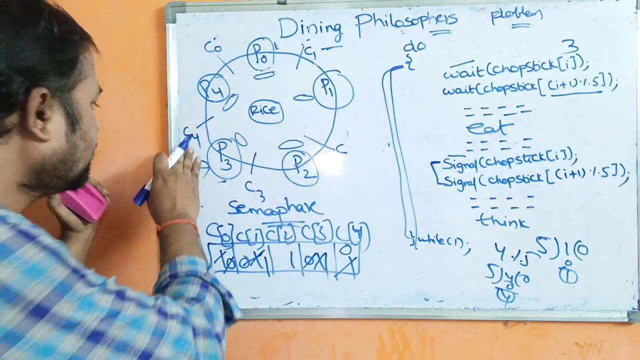 will be changed to zero, will be changed to one now. why? because it is free now. okay, p3 has completed its operation. next signal of chopstick of: i plus one modulo five. so three plus one means what? four four modulo five means four. four modulo five means four. now the c4 is also released. now, this value. 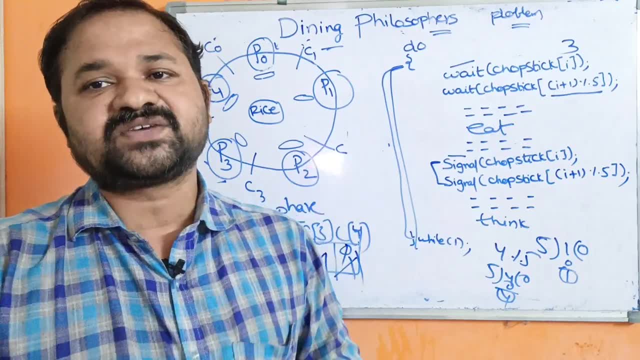 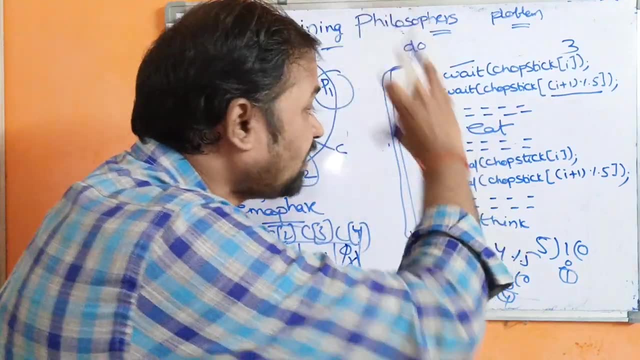 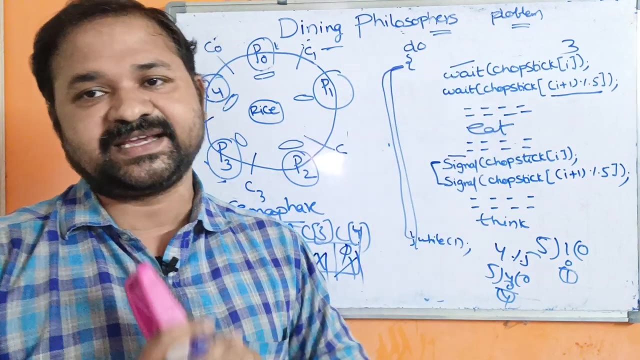 will be changed to one. so, likewise, each philosopher can eat one by one without any problem if he uses this algorithm. but this algorithm will cause us the problem. this algorithm will produce us the dead lock when all the persons wants to eat simultaneously. when all the persons wants to eat simultaneously, then there is a. 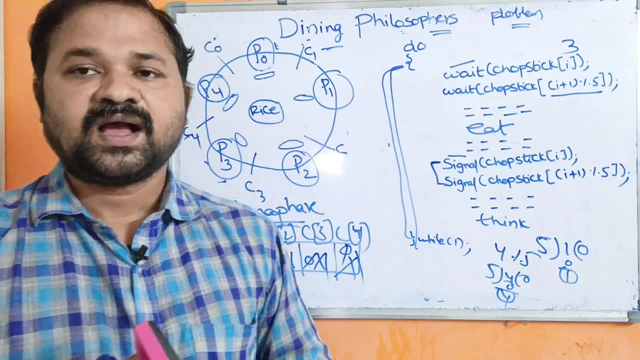 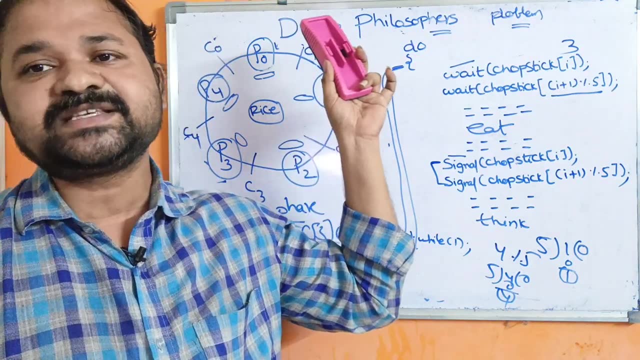 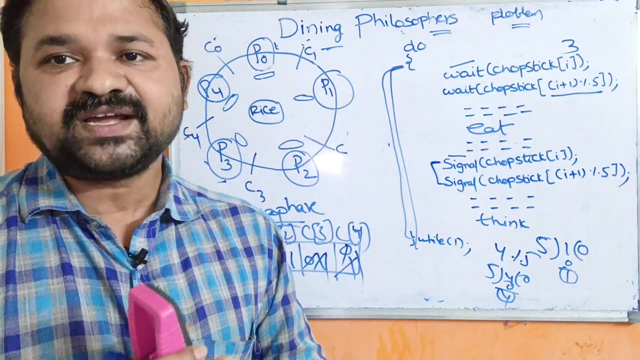 possibility that we may get the red lock already. we have seen that problem. and what is the problem of this algorithm? adjacent philosophers cannot eat simultaneously. while p naught is eating, then p1 and p4 has to wait until p naught completed it's eating okay, so that is the problem. 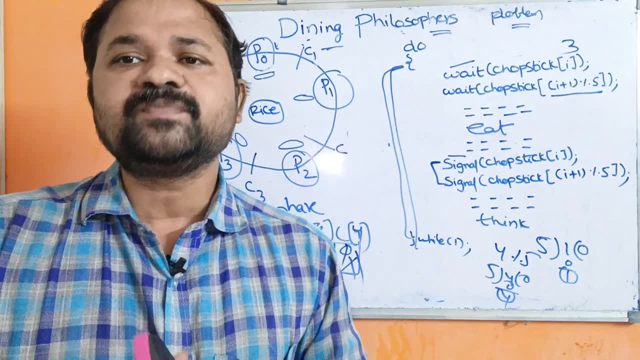 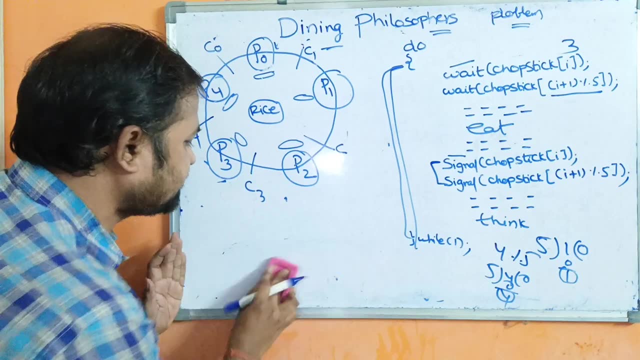 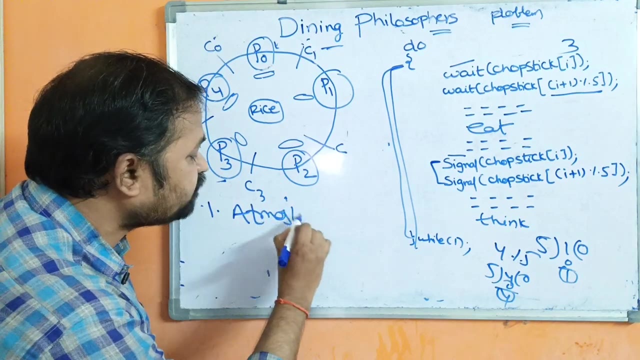 here, so how we can overcome that problem. in order to overcome that problem, we can use three approaches. let us see those three approaches. let us see those three approaches. the first approach is: instead of five philosophers, if we allow at most four philosophers, then this deadlock problem can be. 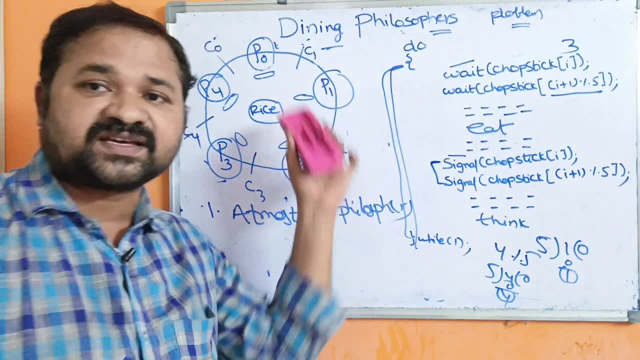 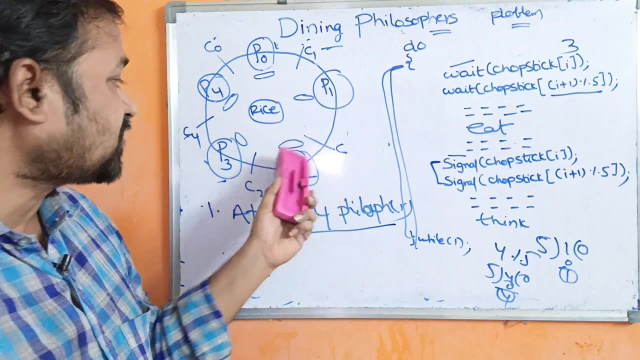 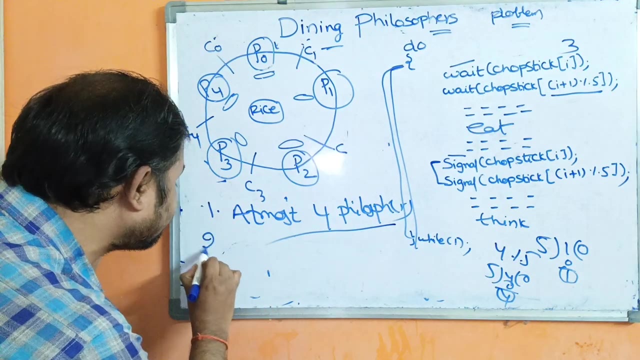 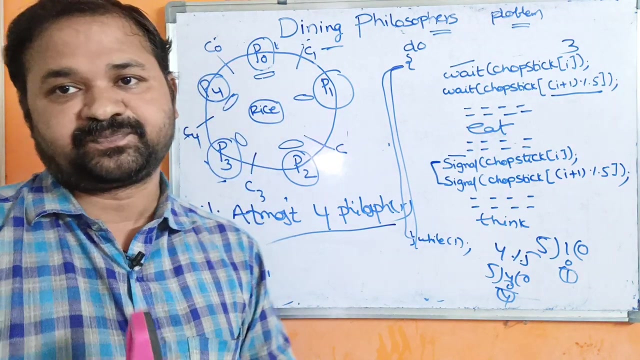 avoided extent. so four philosophers with five chopsticks at most. if we allow maximum four philosophers with five chopsticks, then to some extent we can avoid the deadlock problem. and the second solution is a philosopher has to pick up the two chopsticks only when both are free. so that means 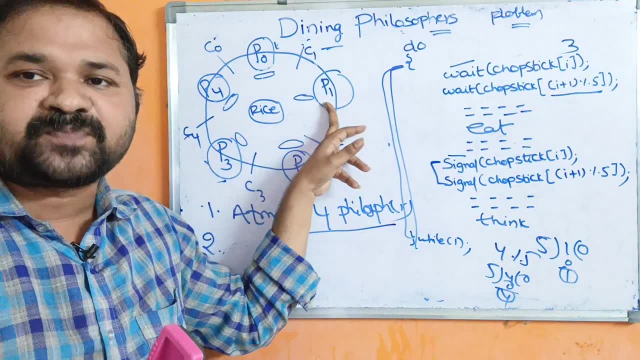 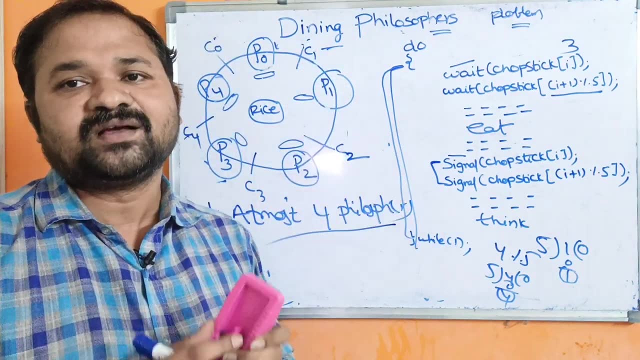 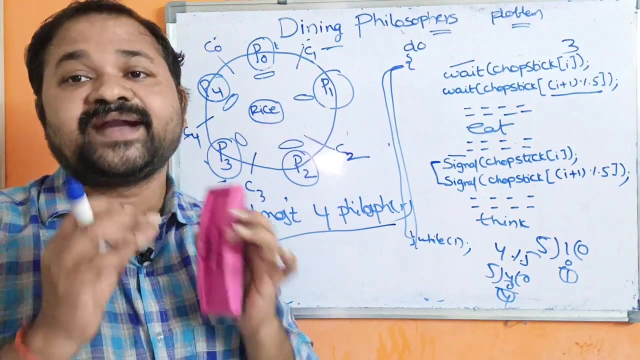 if we consider p1, p1 has to pick up the chopsticks only when c1 and c2 are free. if one of the chopstick is not free, if one of the chopstick is already allotted to some other philosopher, then p1 has to wait until both the chopsticks are free. if we implement this, this approach also, 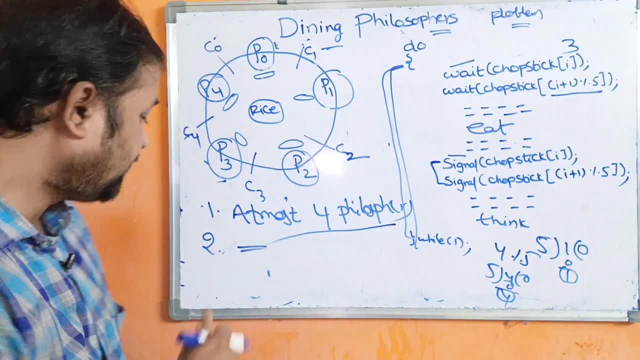 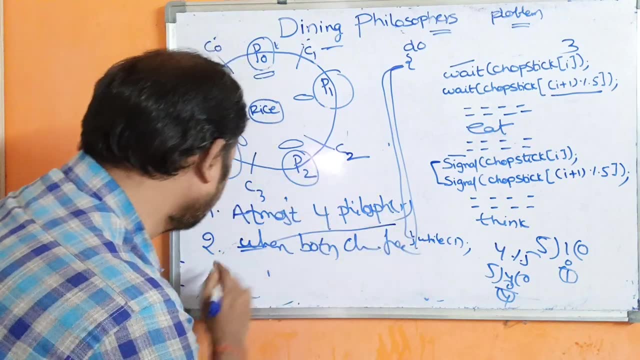 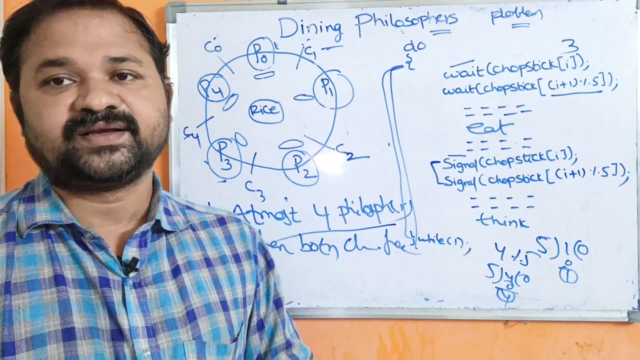 then we can avoid the deadlock to some extent. okay, so when both chopsticks are free, then only the corresponding philosopher has to, has to do the operation, okay. and the last one is: if we change the order? if we change the order, then also to some extent we can avoid the deadlock. so that means